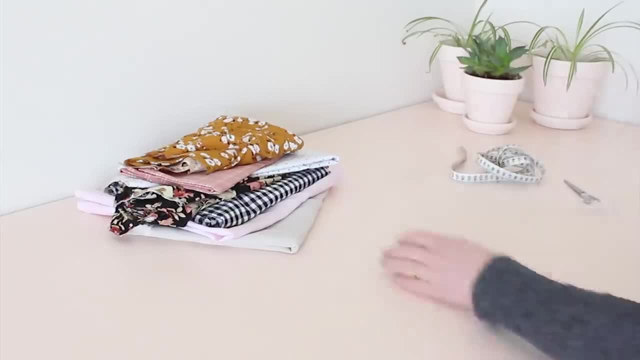 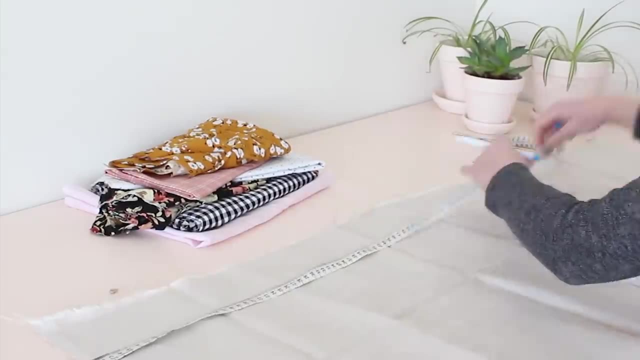 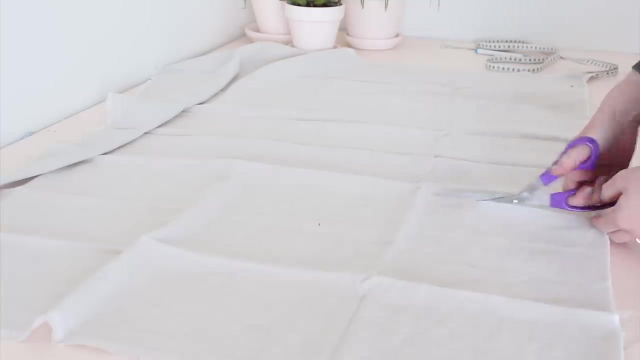 project we're going to make are some lovely linen tea towels. This is a really simple project and a great one for beginners. Start by cutting out a 55 by 75 centimeter rectangle from your linen fabric. I'm using my water erasable pen to mark the rectangle out before cutting Linen is one. 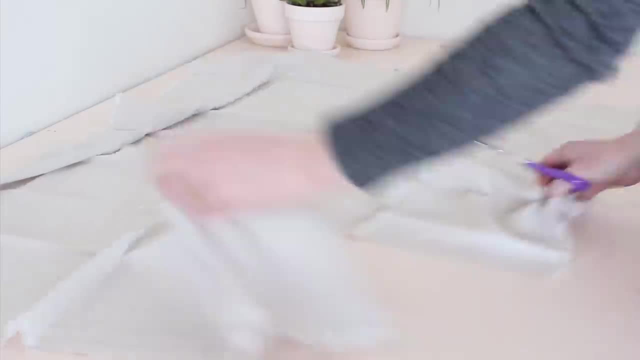 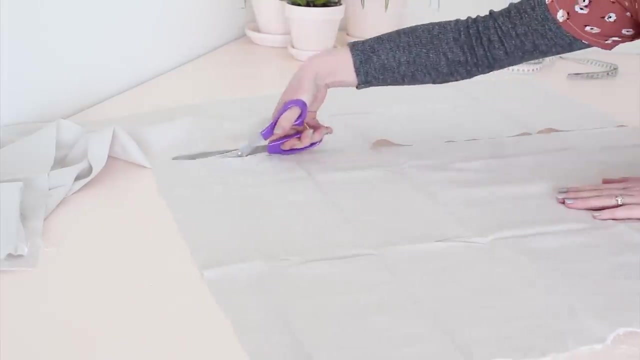 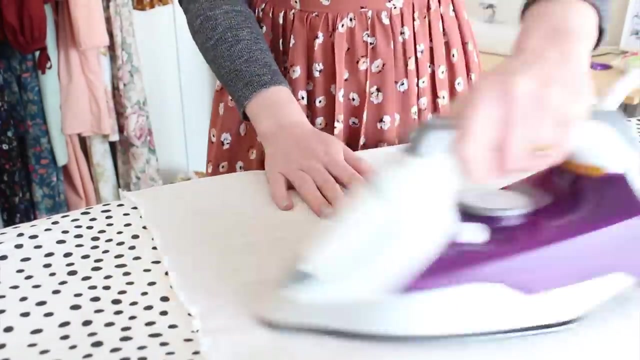 of my most favorite fabrics to work with and it's quite easy to get a hold of. You should be able to find it in most fabric stores. Next, iron out some of the creases- Linen does crease pretty easily, by the way- and then hem the. 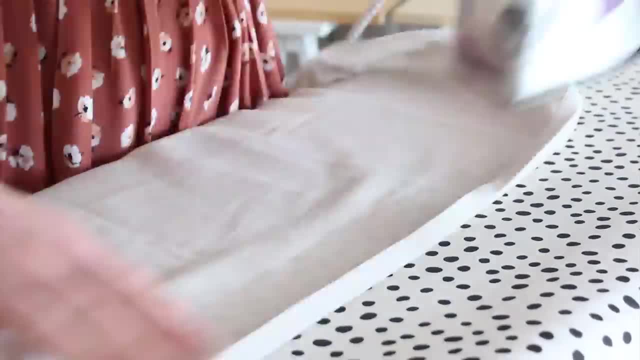 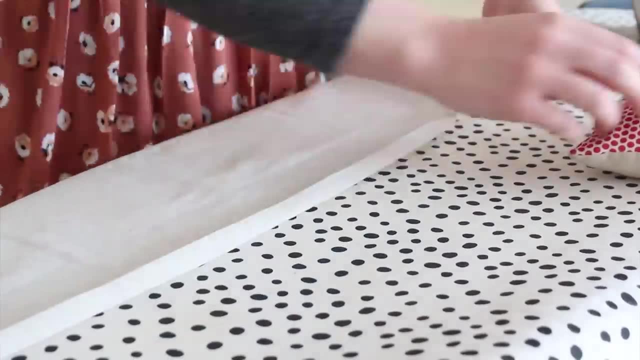 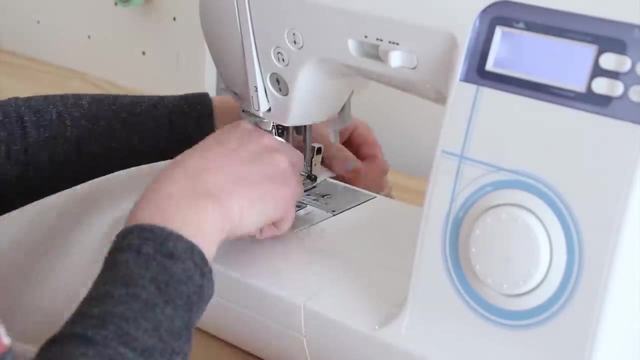 two longer sides of your tea towel by ironing and pinning in place. Stitch the hem down. To keep the stitches straight, I like to line the sewing machine foot up with the edge of the fabric. Next, head back to the iron and hem the two. 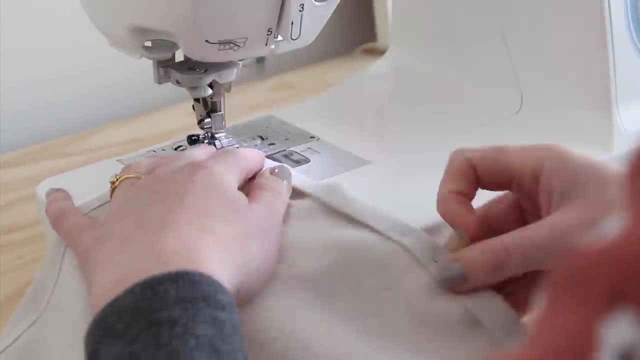 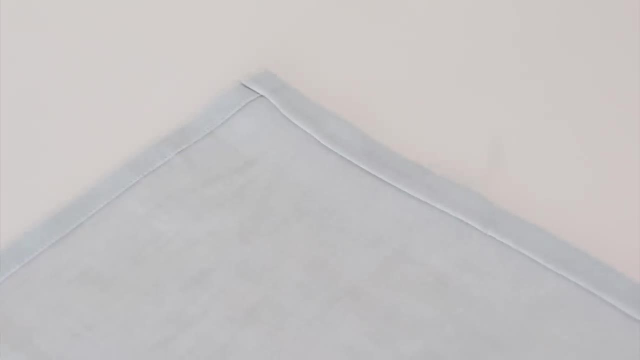 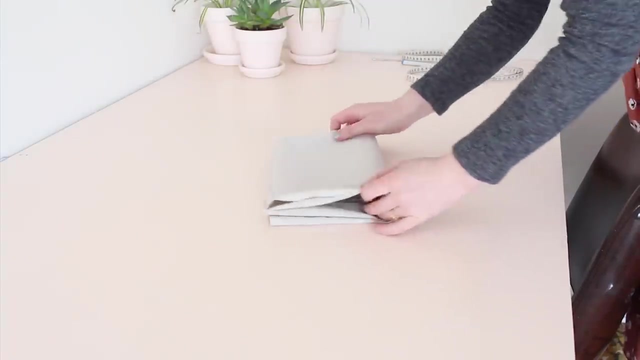 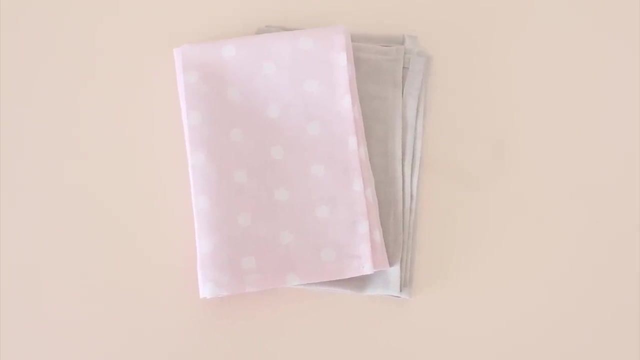 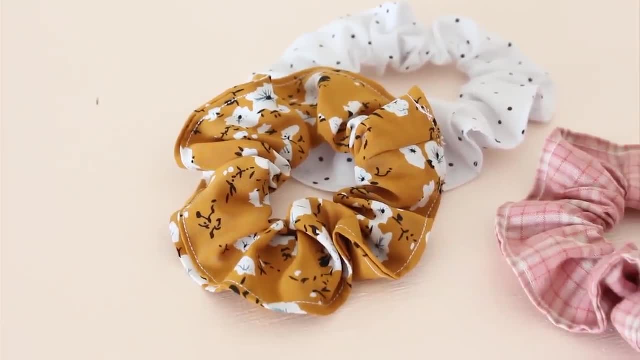 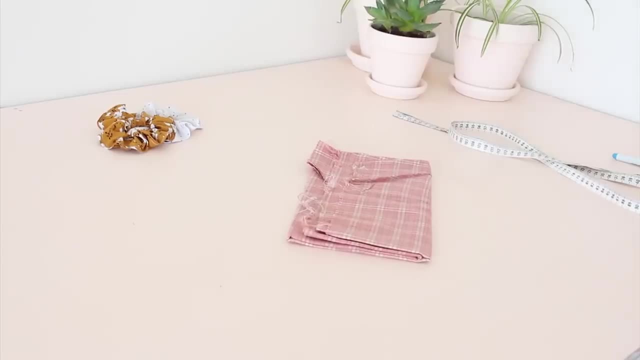 love making scrunchies from my scrap fabrics and I like to pop them in with every order from my online store, so it's fair to say I've made a fair few over the years. To make one for yourself, cut a 50 by 10 centimeter rectangle from your. 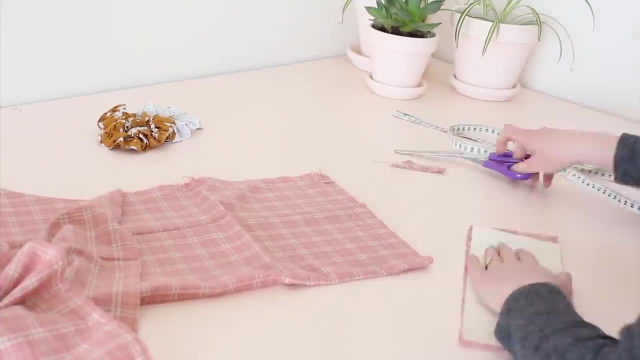 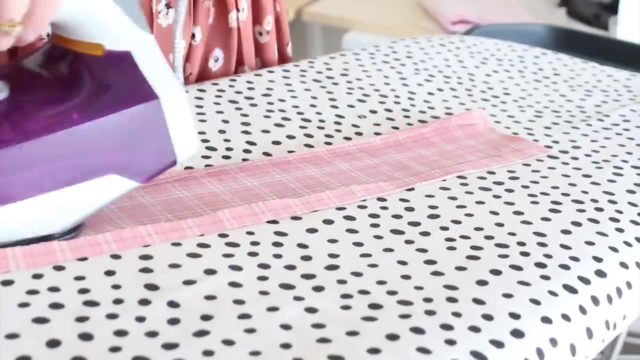 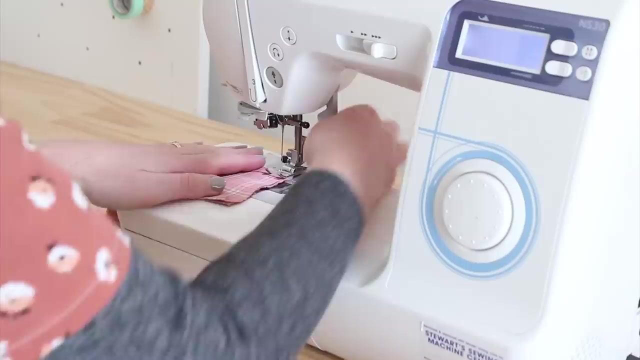 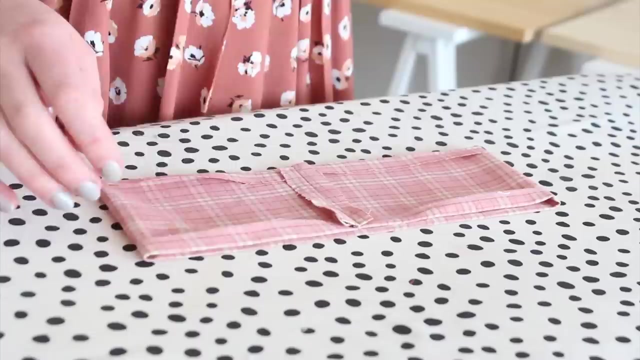 fabric. Next, fold the two longest edges in about one centimeter and iron flat. Then fold your fabric in half at the middle with the folded edges visible from the outside. Sew the fabric at the raw edge to create a kind of loop. Iron the seam flat. then fold the loop in half, wrong sides together, meeting the. 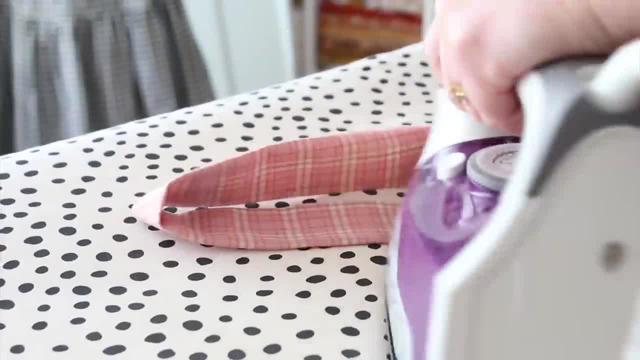 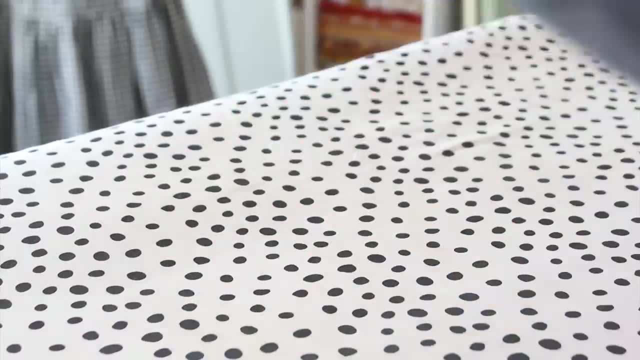 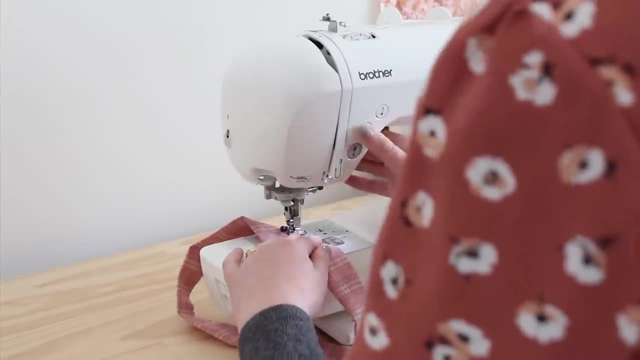 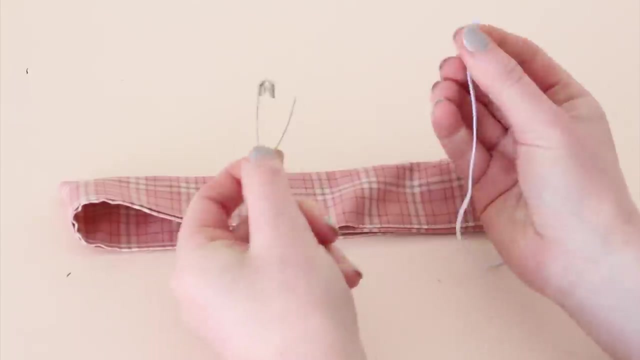 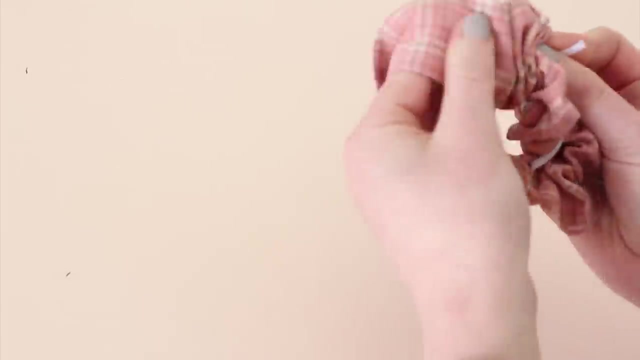 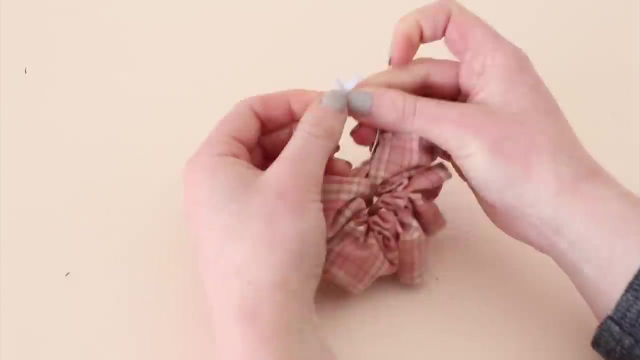 two folded sides together. Sew the folded side together, leaving a small opening at the end to thread the elastic through. Next, cut a 20 centimeter piece of elastic Using a safety pin, thread the elastic through the fabric casing, Tie the elastic together with a triple knot and sew the. 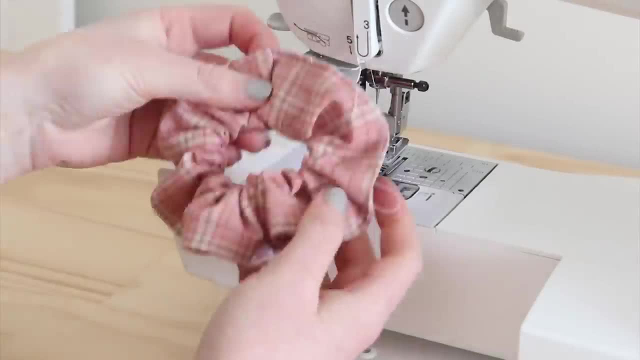 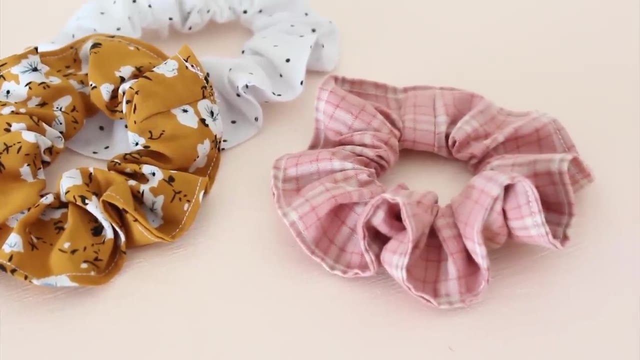 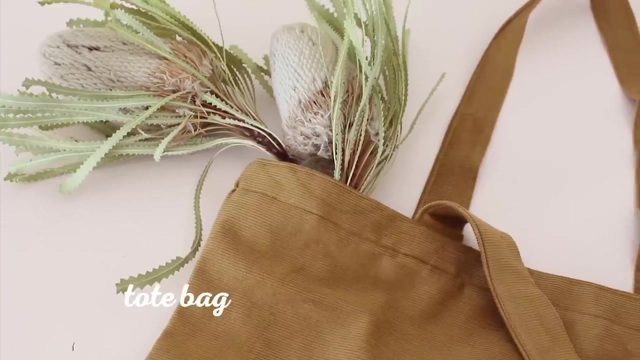 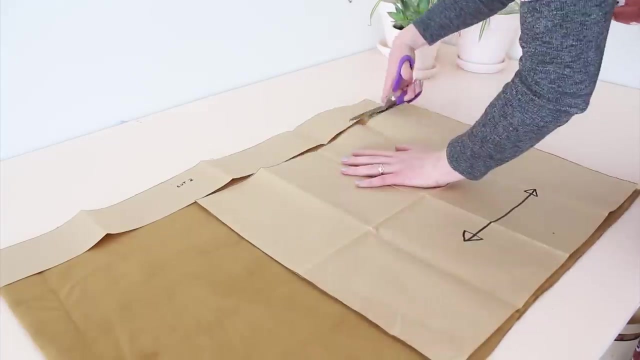 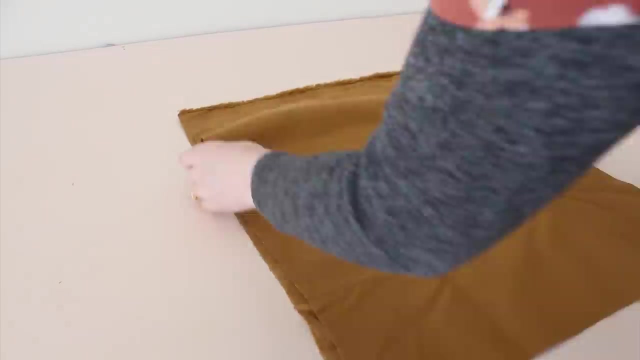 small opening closed. Now let's make a super useful tote bag. Start by cutting out two 50 by 45 centimeter rectangles and two 80 by 8 centimeter rectangles with right sides together. pin the two larger rectangles together along all sides except one of the. 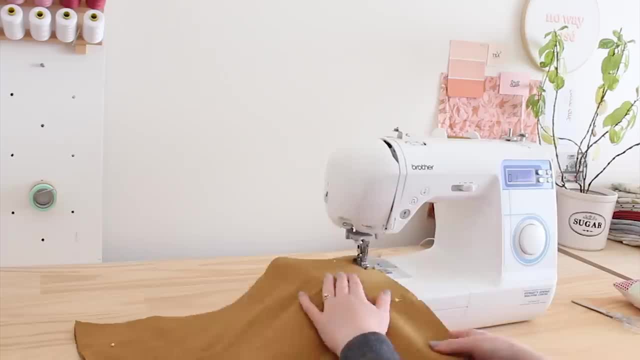 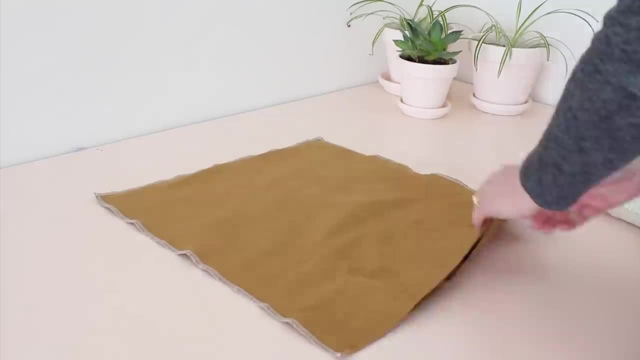 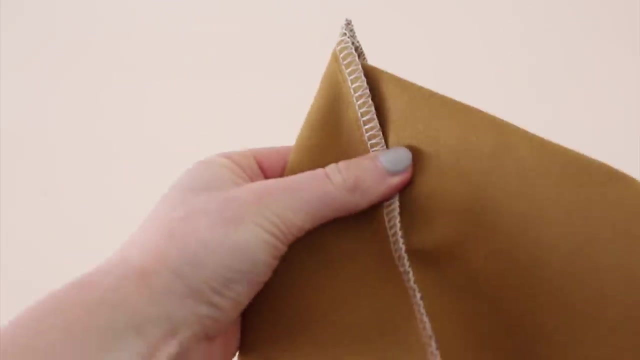 shorter sides. Sew along the three sides and, if you have one, overlock the raw edges. Next, fold the bottom corner of the bag together, pinning approximately 7 centimeters from the top of the point. Sew along where you've pinned, obviously. 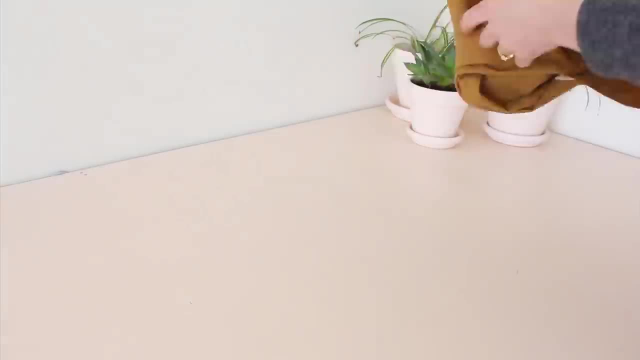 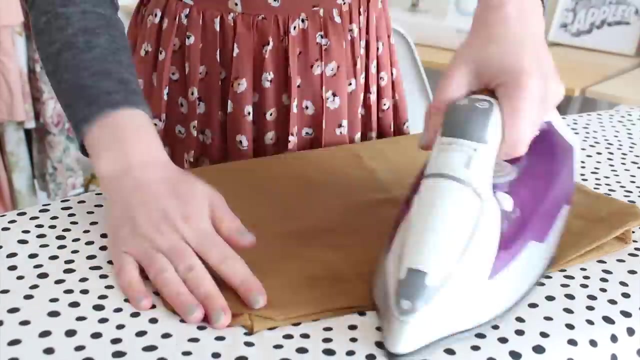 removing the pin as you sew. This step creates a sort of fold in the bag, giving it a little bit of extra room at the bottom to carry more around in. To finish your tote bag, hem the top of the bag by folding in approximately 2.5. 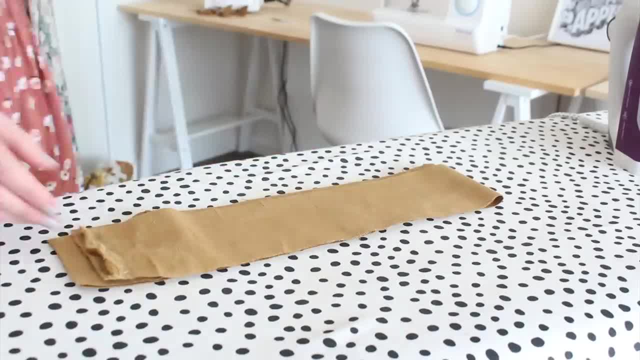 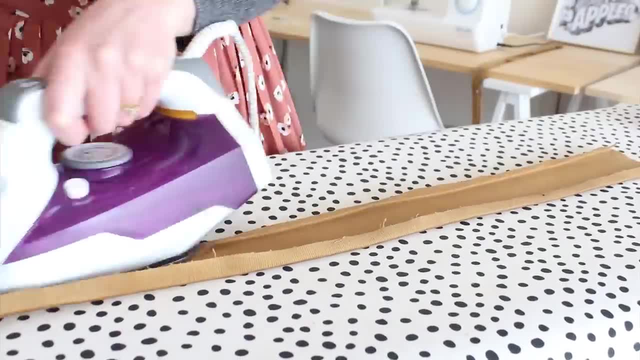 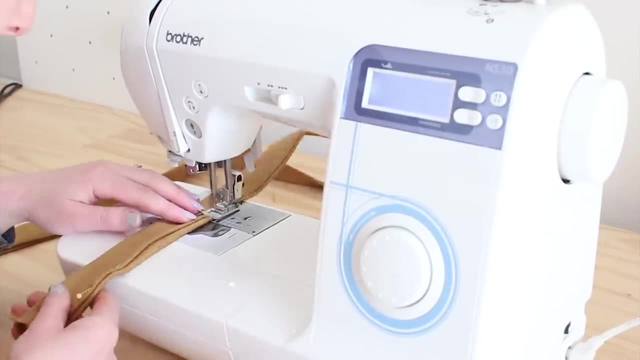 centimeters twice. Take the two long rectangle pieces and fold the two longest edges in about one centimeter and iron flat. Then fold the rectangle in half long ways meeting the two folded edges together, and iron this flat too. Then sew all along this folded edge. 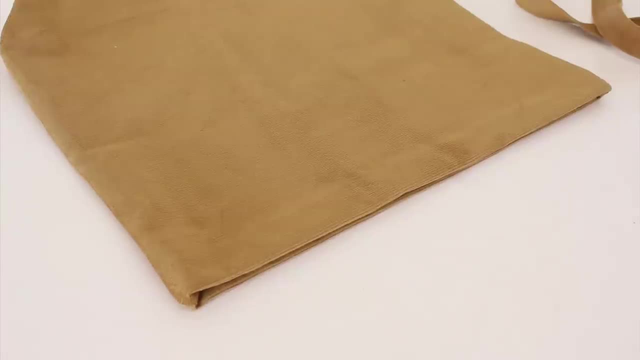 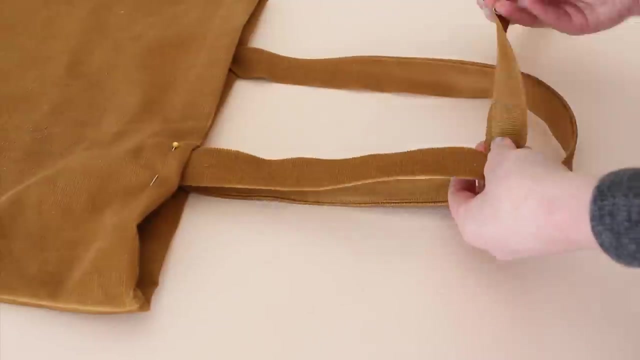 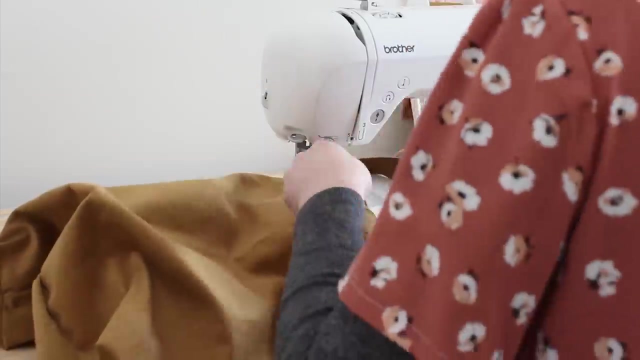 Once your handles are done, place them in the folded edge of the bag and pin in place. Pin the other handle on the other side, making sure they are pinned in roughly the same place. Stitch along the folded edge of the bag, making sure to stitch the handles down securely as you sew. 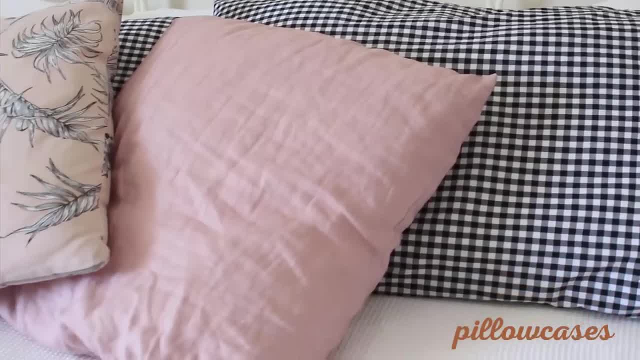 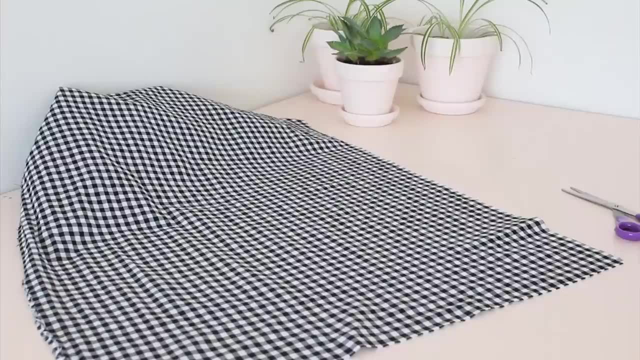 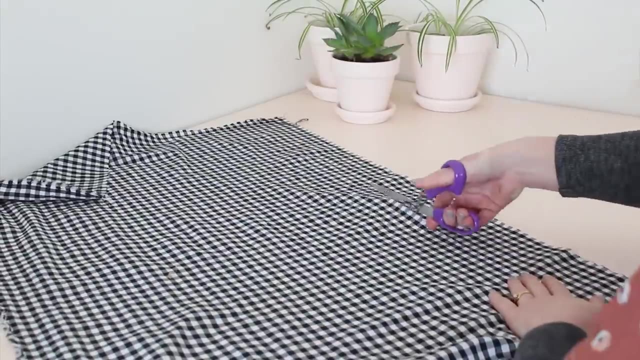 This next project I'm really excited about and I didn't realize just how easy they were to make. Let's make some pillowcases. Start by cutting a 160 by 50 centimeter rectangle from your fabric of choice. I've used some gingham for mine. 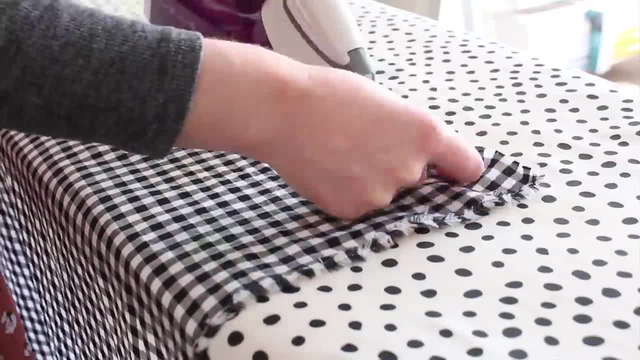 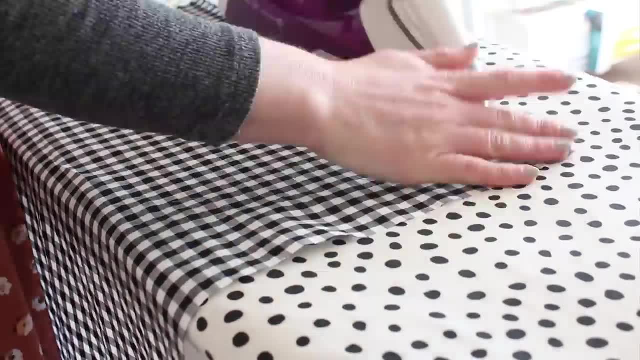 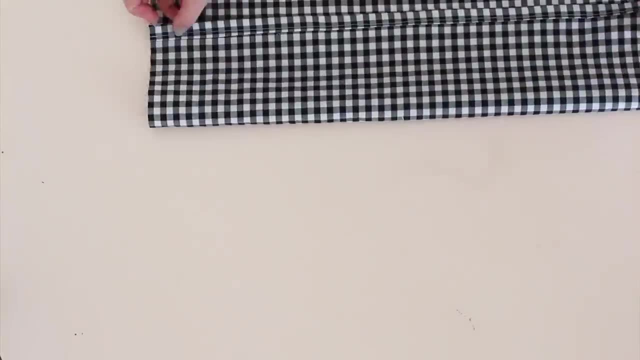 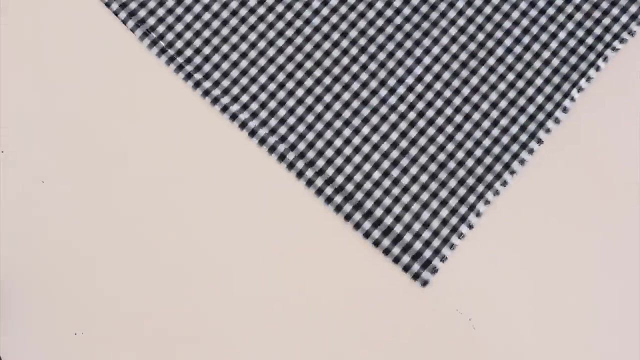 and I'm in love with how they've turned out. Next, hem the two shortest edges by ironing and pinning, then sewing in place. Fold one edge of the pillowcase in by about 13 centimeters. Then, with right sides together, fold the pillowcase in. 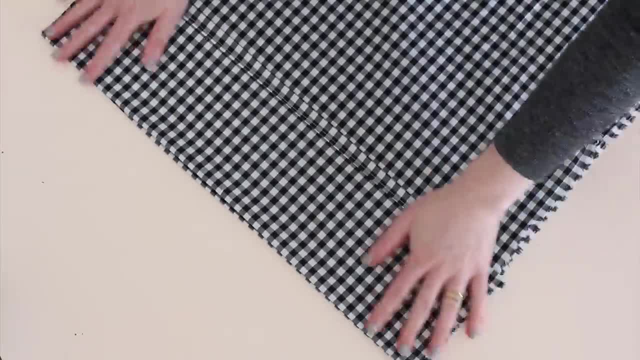 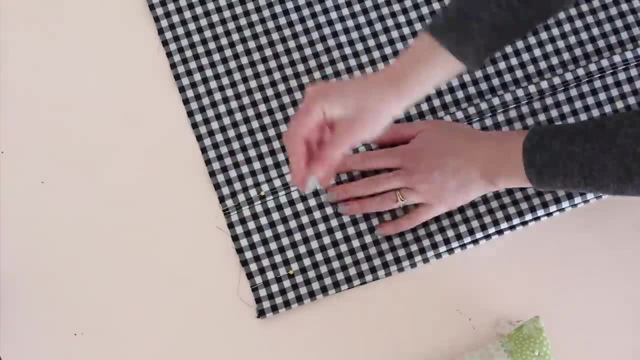 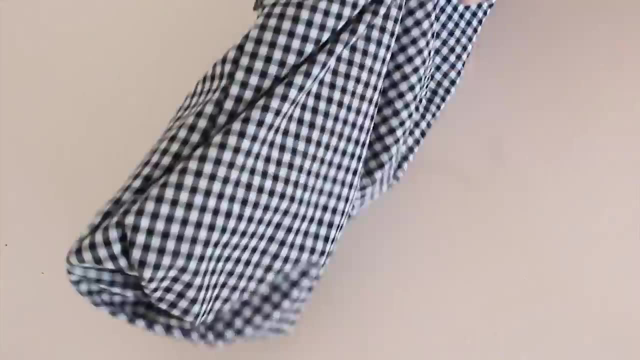 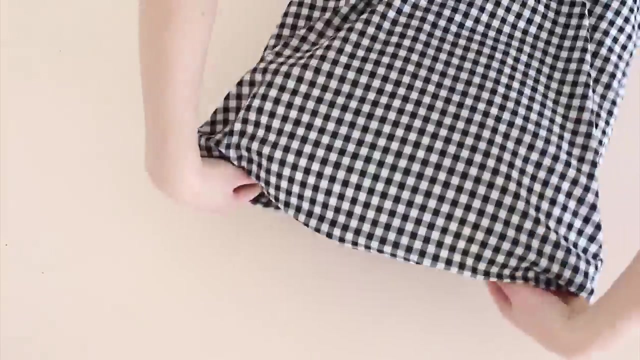 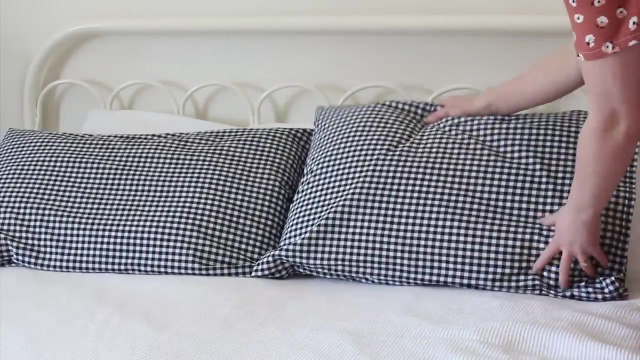 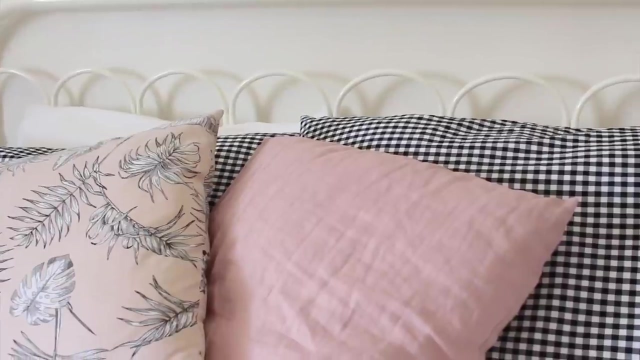 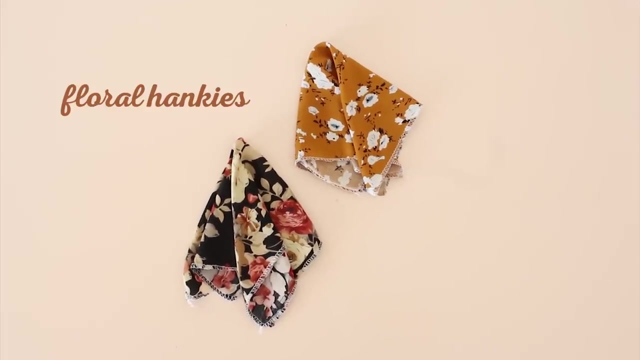 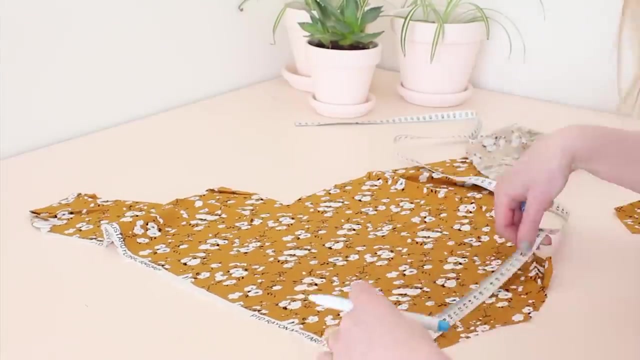 half meeting the folded edge and the hemmed edge together. Pin along the two longest sides and sew in place. Fold the, Fold the pillowcase right side out and pop your pillow inside. And now for the last project: floral hankies. These are so quick and easy to make, but you'll need an overlocker to make these cute hankies. 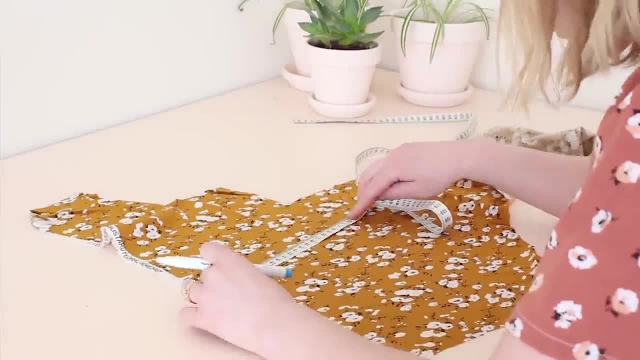 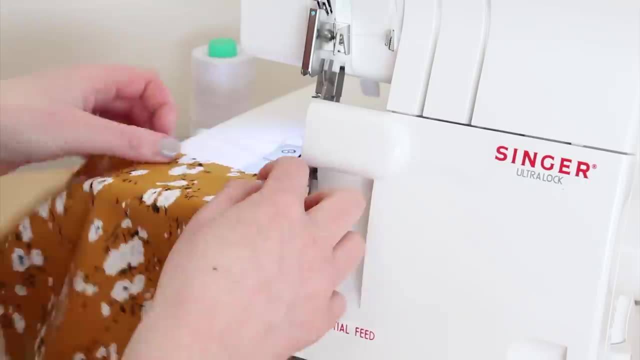 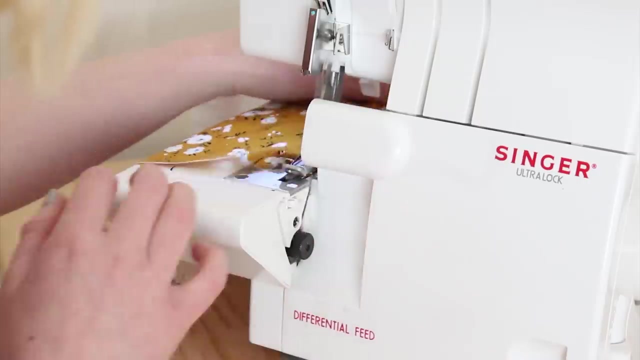 Start by cutting out a 22x22cm square of fabric. It doesn't have to be floral, but floral fabric does make for a really cute hankie. Next, set up your overlocker for a rolled hem. I share how to make a rolled hem and how to set up your overlocker for one in a previous 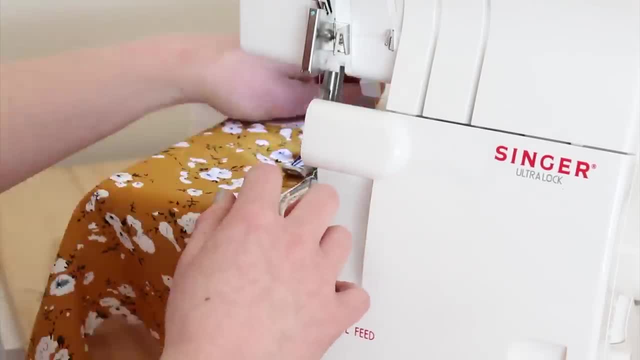 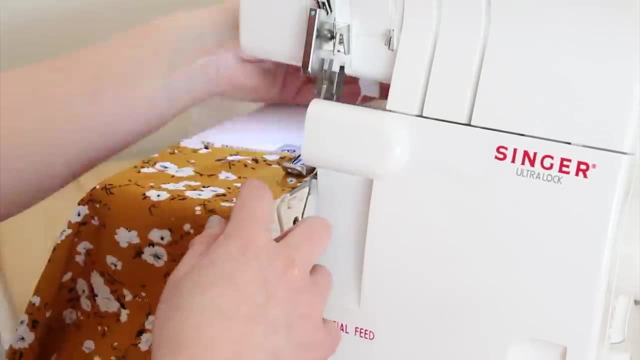 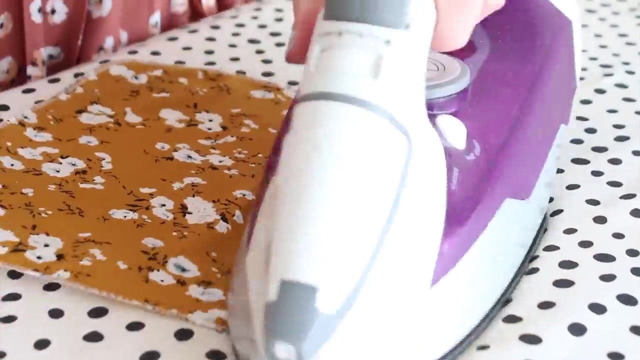 video, so I'll leave that link down below. if you'd like to find out how, Then, simply do a rolled hem, stitch along each side of your fabric square. Once sewn, cut the stitch chains off and press the stitches with an iron.